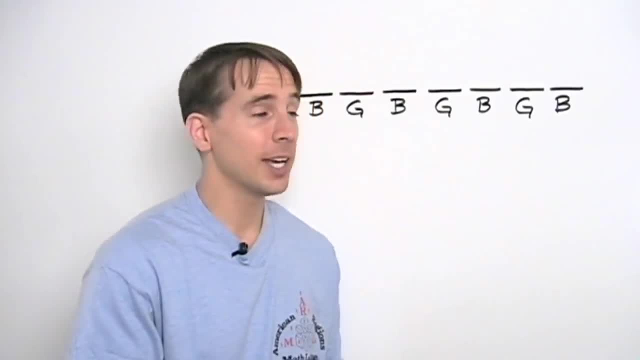 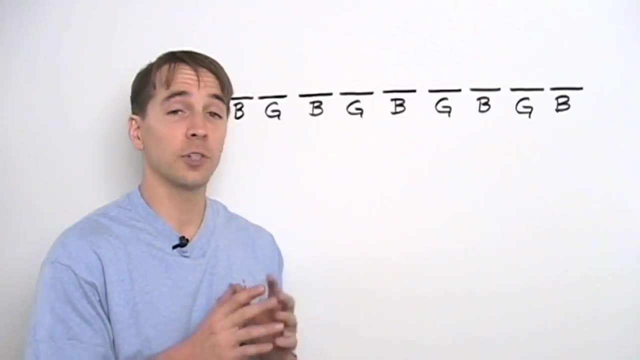 and it's a problem. I like twice as much as most counting problems. Well, here's the problem. She was taking her class to a play for the first time. It was the first time she ever took the whole class somewhere and she was worried, You know, she'd bring them to the playhouse. She's. 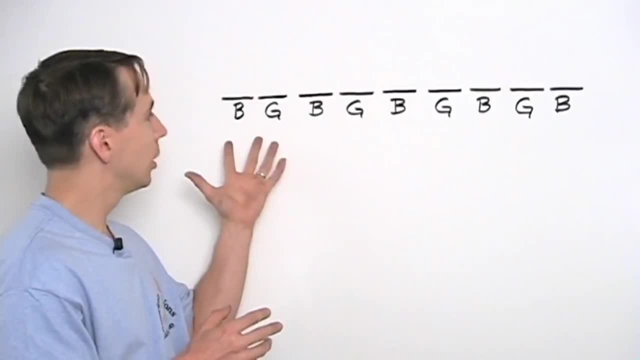 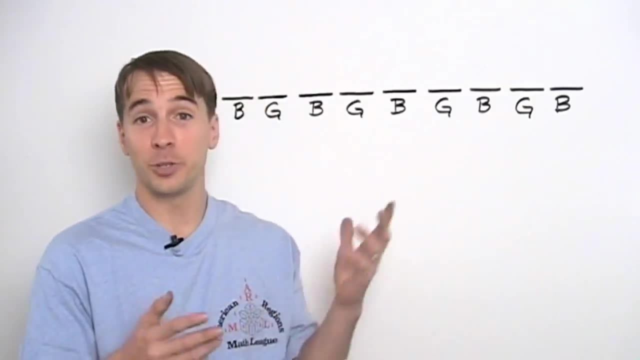 worried the kids would talk, They'd be loud during the performance. So what she did was this: She had the kids seated: boy girl, boy, girl, boy girl. Now we all know this wouldn't work in middle school, wouldn't work in high school, but back in first grade, you know the boys and the 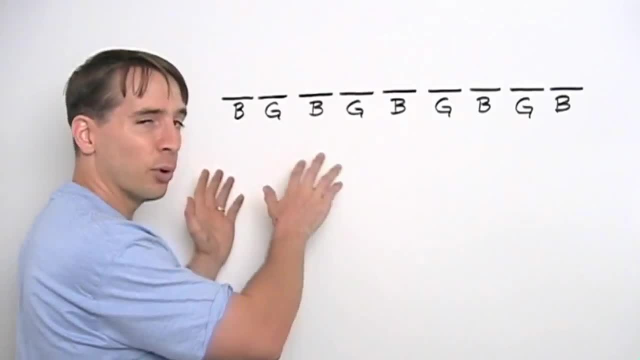 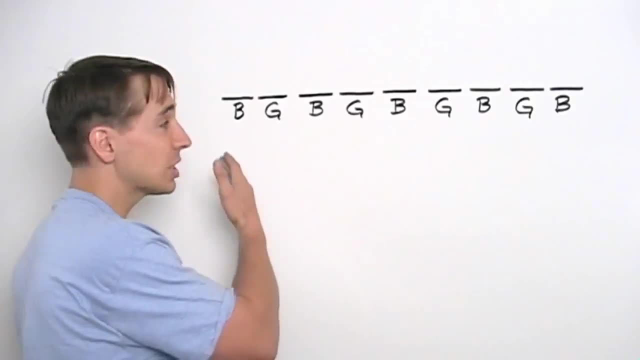 girls believed in the whole cooties thing. So you know, sitting in boy girl, boy girl, a lot less talking than if you have all the boys together and all the girls together. So she told the ticket person: just hand out seats one, three, five, seven, nine. 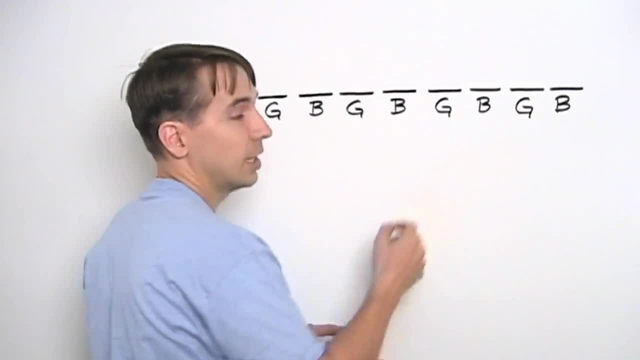 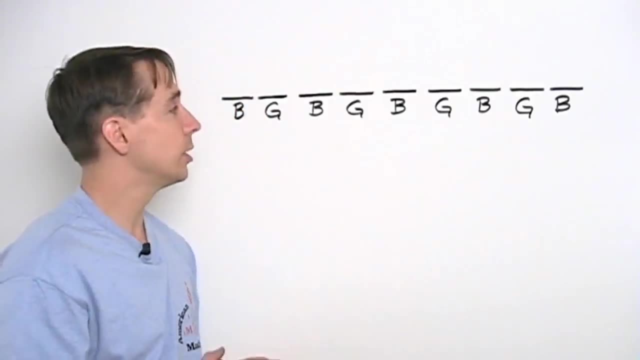 Walking to the boys at random and seats two, four, six, eight to the girls at random, And she had five boys and four girls there, So the ticket person handed out the tickets completely at random to boys and girls, just like this. The odd numbers went to boys, Even numbers went to girls. 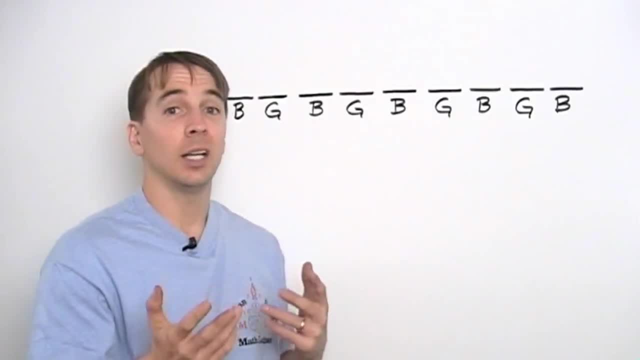 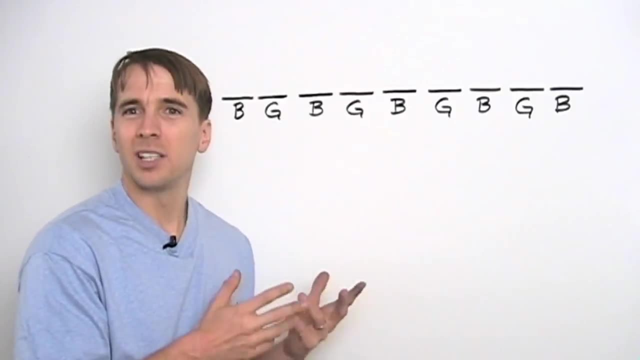 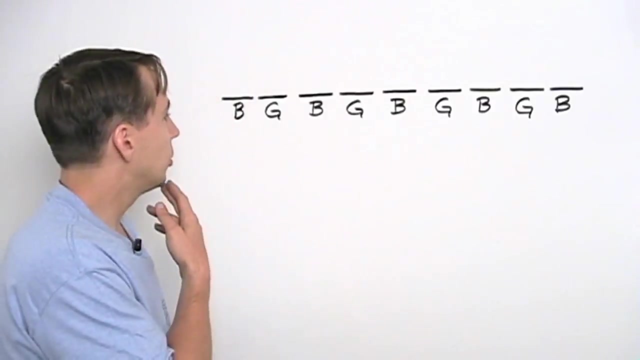 Then my mom realized, as the kids were walking to their seats, she had a brother and sister in the class who were very, very shy and they were new to the school. So well, they might be more shy than the boys, but the kids had already been given out and the kids were headed off to the seat. 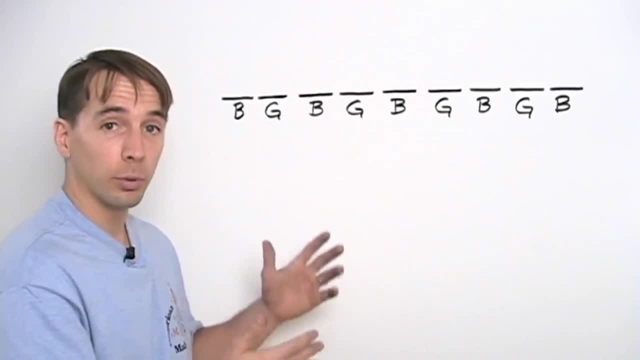 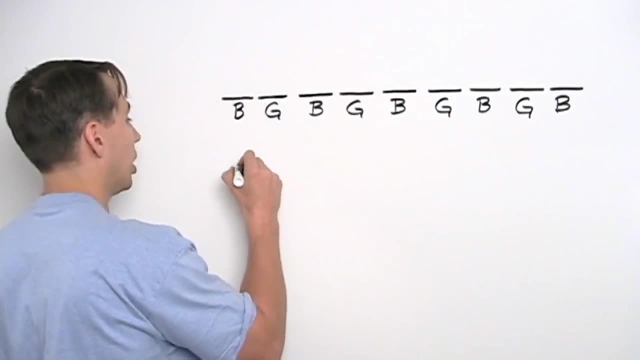 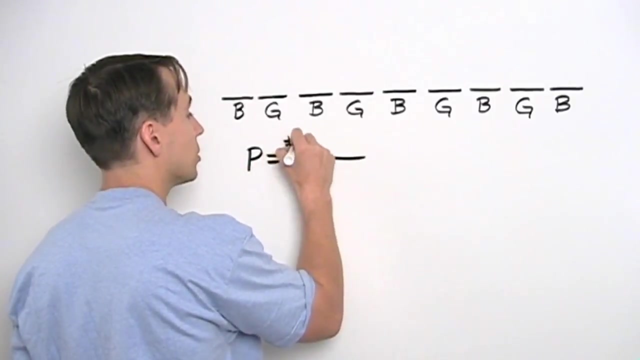 So here's the question: What's the probability that the brother and sister ended up together? And we're going to go after this problem the way we do a lot of probability problems. Our probability is the number of successful outcomes, That's, the ones where the boy and the girl, brother and sister. 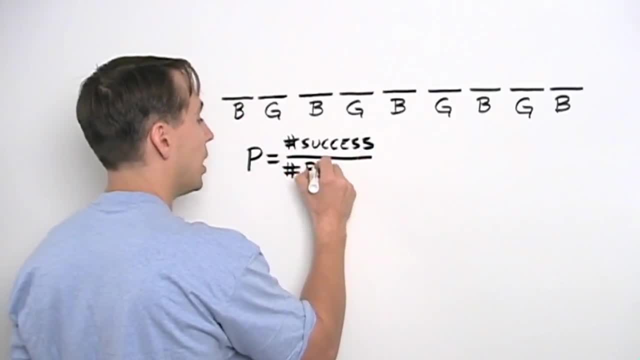 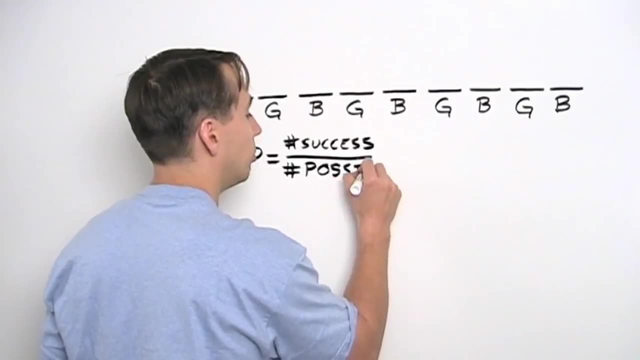 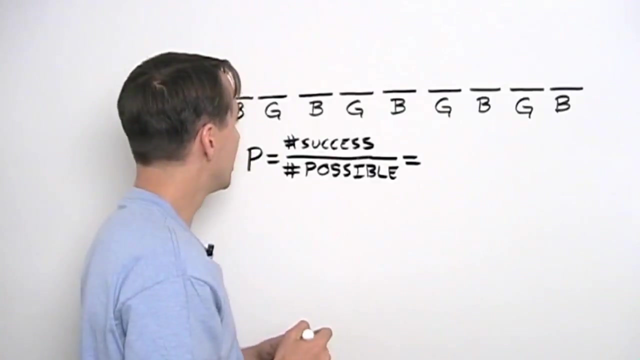 and we're going to divide by the number of equally likely possible outcomes And we have our possible outcomes laid out right up here: Boy girl, boy, girl, boy girl. And now you see why I like this problem two times as much as most counting problems, because now we have two counting problems. 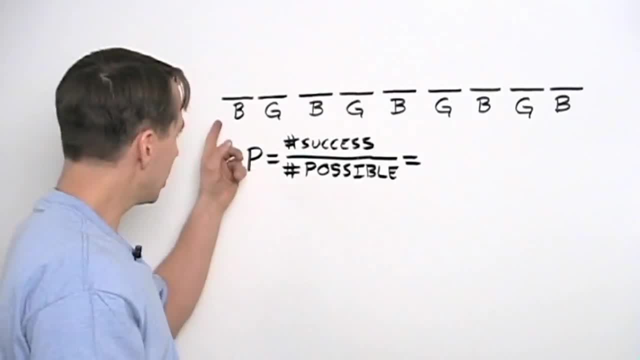 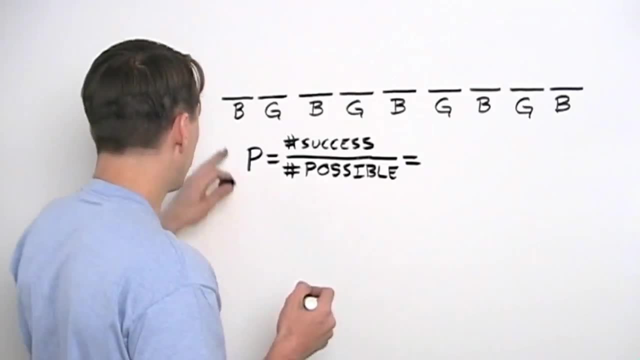 First we have to count the number of possible outcomes. How many ways could the tickets have been given out? boy girl, boy, girl, boy girl. Well, let's deal with the boys first, This first ticket. there are five boys, so there are five ways this ticket can be given out. 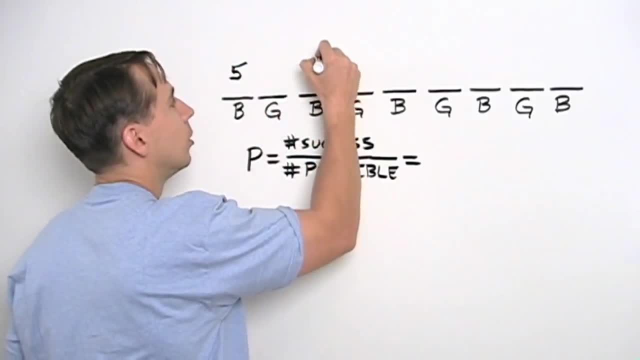 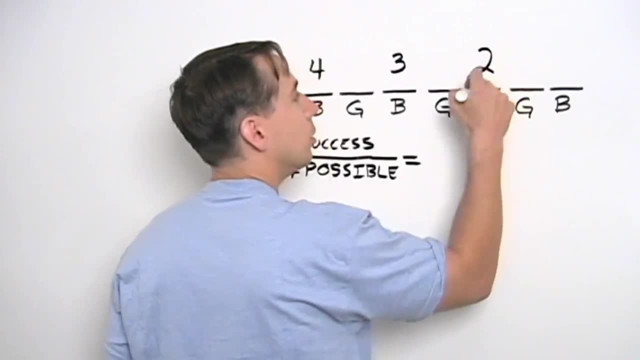 And after that ticket is given out, well, there are four boys left to get the next boy ticket, and there are three boys left to get the next boy ticket, two boys left to get the next to the last one, and then there's only one boy left without a ticket. 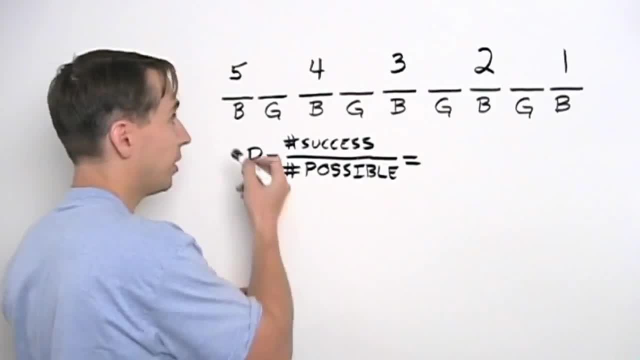 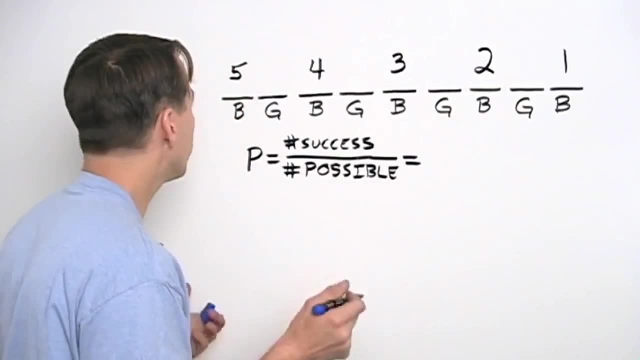 He gets the last ticket. So you see there are five factorial five times, four times, three times, two times, one ways to give out the boys' tickets. And for the girls it's pretty much the same thing. There are four girls, so there are four choices for the first of the girls' tickets. 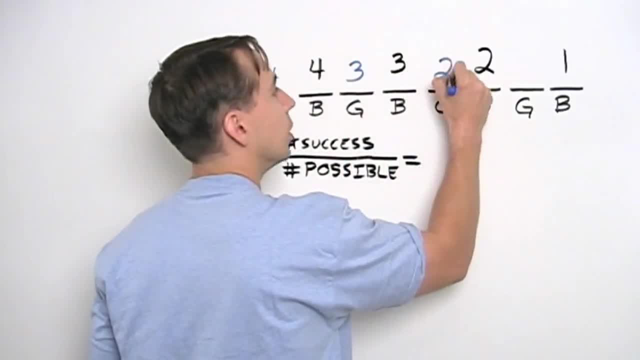 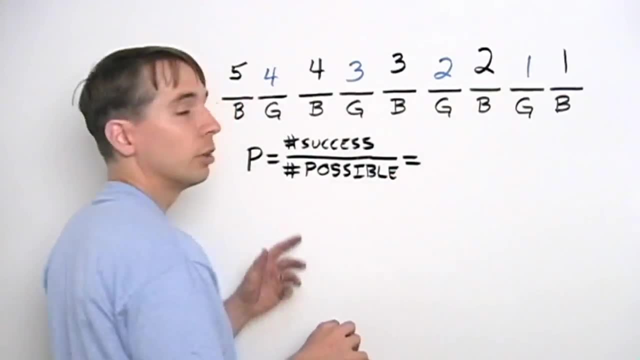 That leaves three girls for the next ticket, two for the next and one for the last. So you see that for each of the five factorial ways to give out the boys' tickets, there are four factorial ways to give out the girls' tickets. 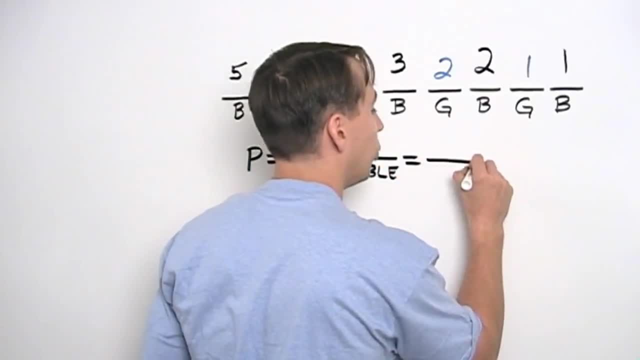 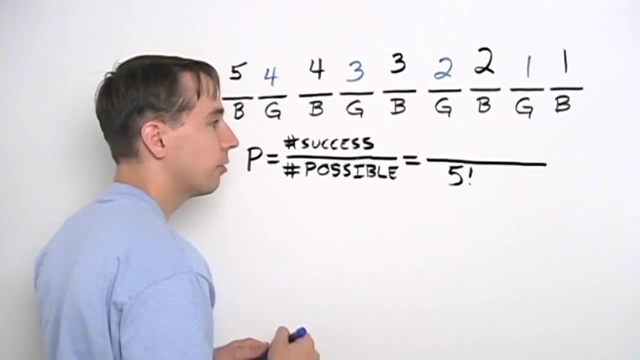 So now we know there are five factorial ways, So times four factorial possible ways to give out the tickets. I'll go ahead and keep with my black for the boys and blue for the girls. So we've counted our total number of equally likely possible outcomes. 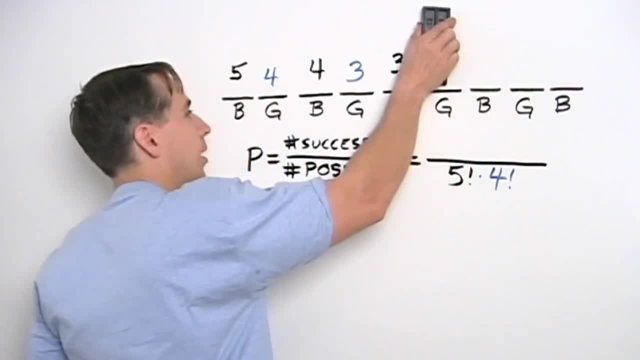 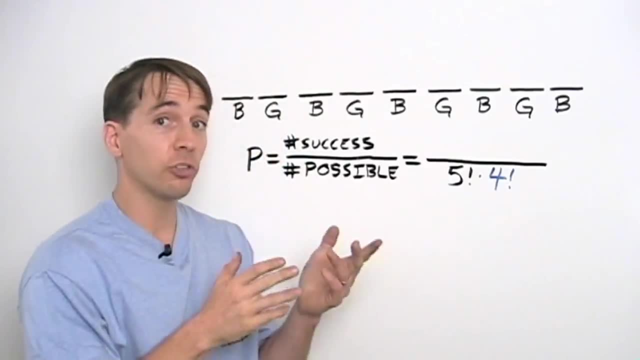 Now we have to count the successes, And that, of course, is another counting problem. But this is a counting problem with a special restriction. The brother and sister have to sit together And we know how to handle counting problems with special restrictions. 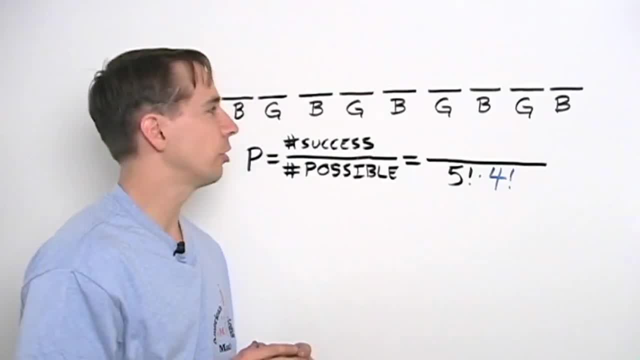 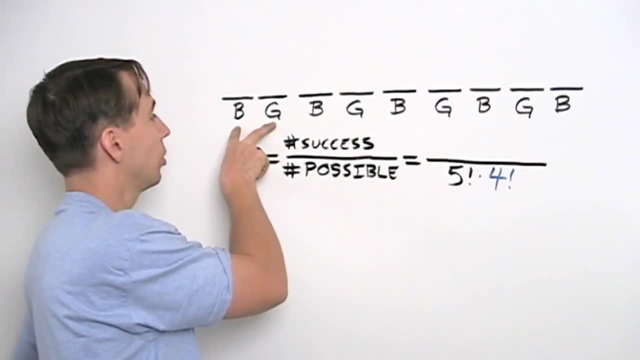 We usually focus on the restriction first. So here we'll focus on the brother and the sister And we'll go ahead and seat them first. Now, if we seated the brother first, or if we put him in the first seat, the sister would only have one option. 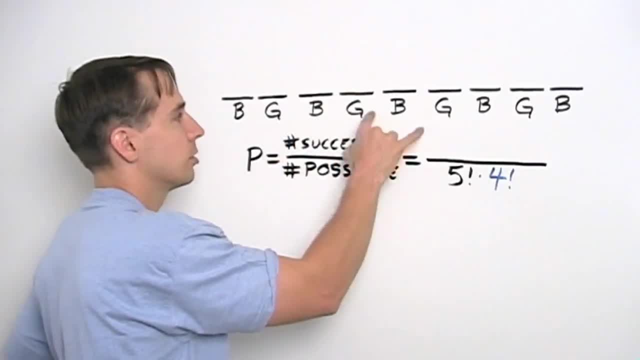 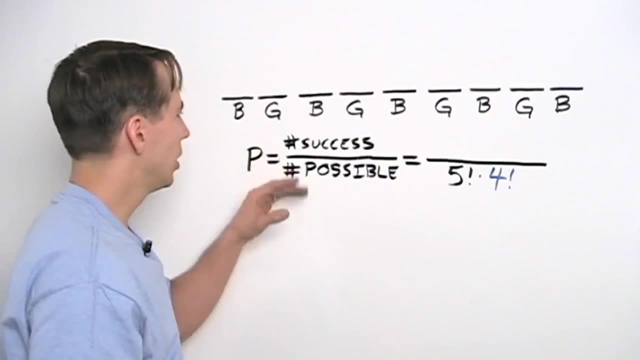 But if we put him here, the sister has two options. Here sister has two, Here sister has two, Here sister only has one. I could send this into some casework. Nobody likes casework. So let's think about what happens if we seat the sister first. 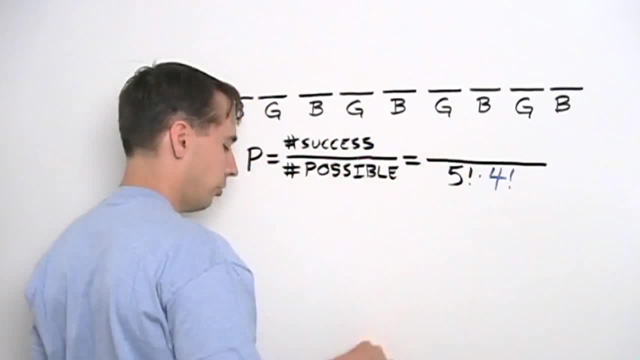 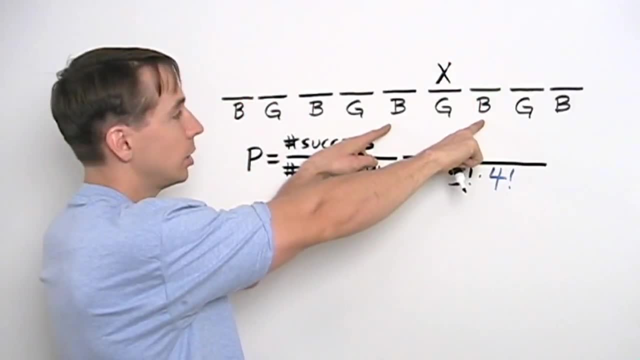 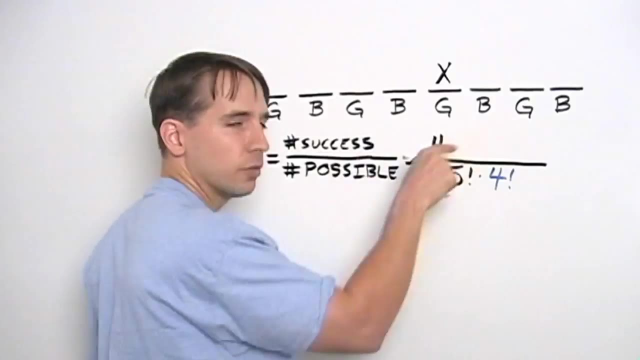 We seat her in any one of these four girl slots, Say we put her right here, Then the brother has two choices, Either of the slots next to her. So the sister has four choices And no matter which of these four she takes. 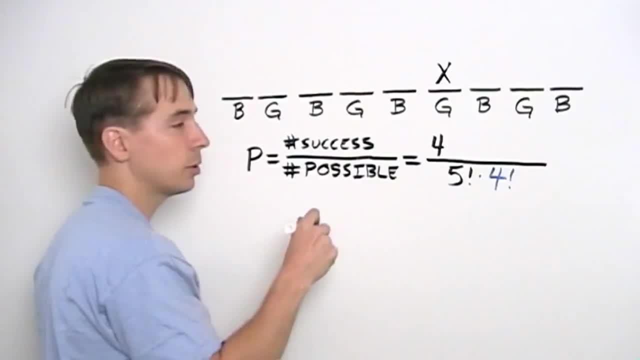 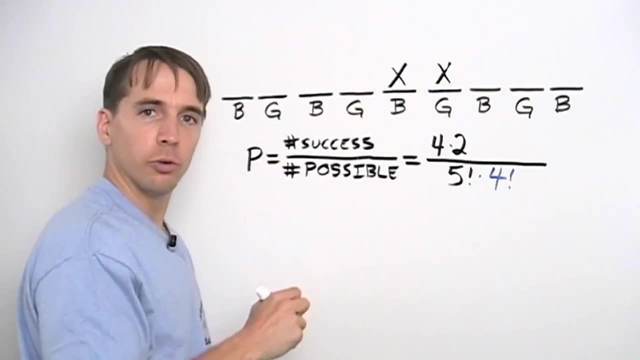 brother has two choices: two seats next to her, Because there will always be two seats next to her. So let's say he takes this one Now, once those two have been placed in their seats. well, now the rest of the problem is just like what we did. 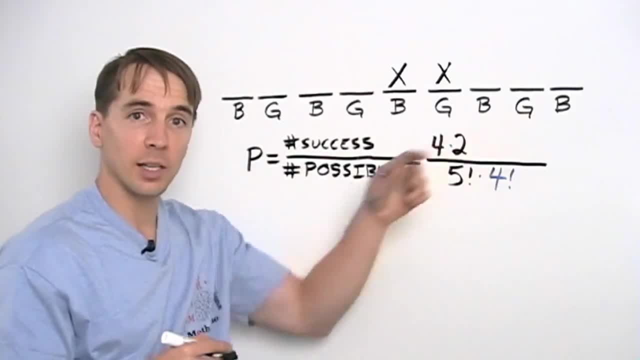 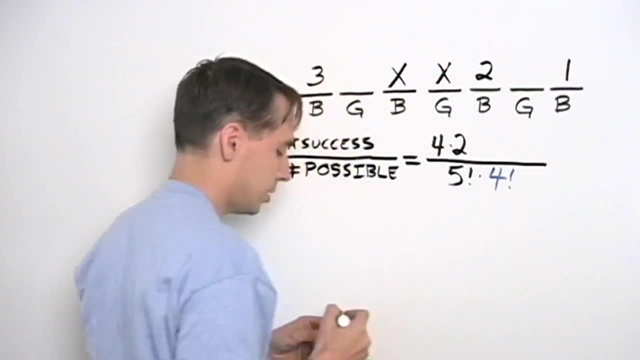 with the number of possible outcomes. We have four boys left. There are four tickets left, So there are four ways to give out: the first ticket, then three for the next one, two for the next one, one for the last, And then pretty much the same way. 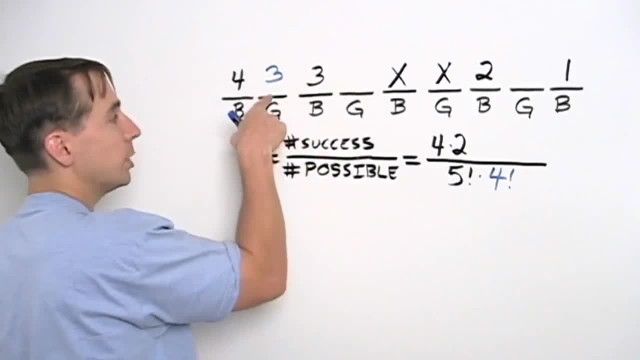 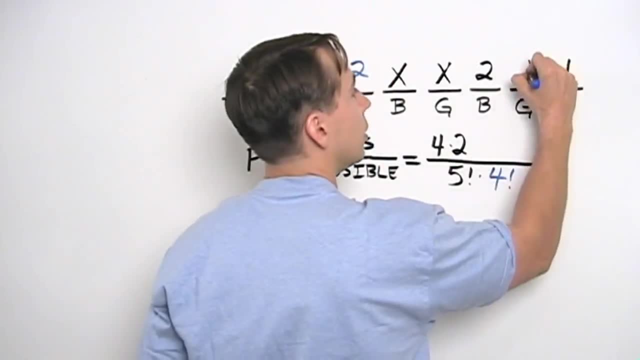 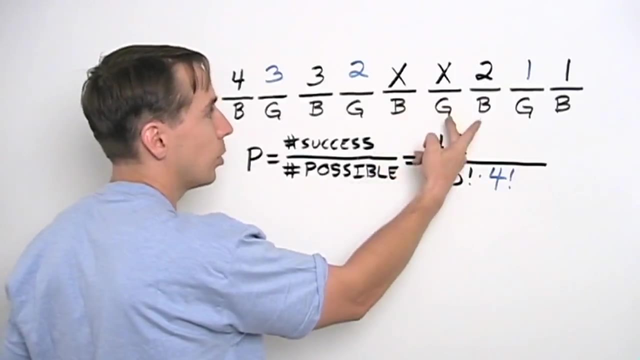 the same thing with the girls. There are three tickets left, Three girls left for this spot, There are two girls left that could take that spot And one girl left for that slot. So for each of the four times, two ways that we can seat the brother and the sister. 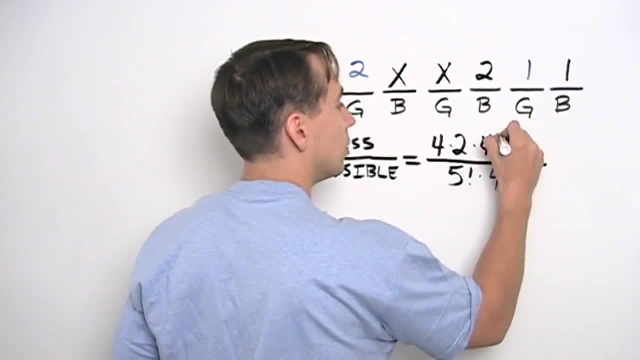 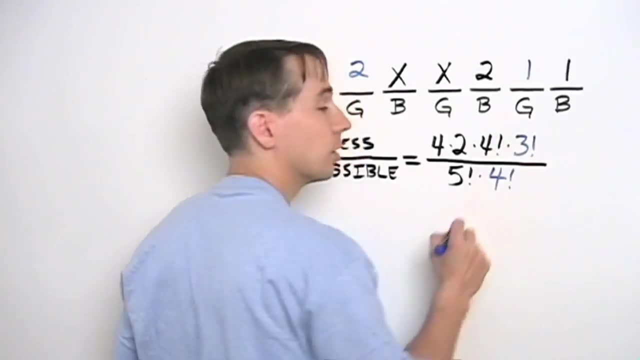 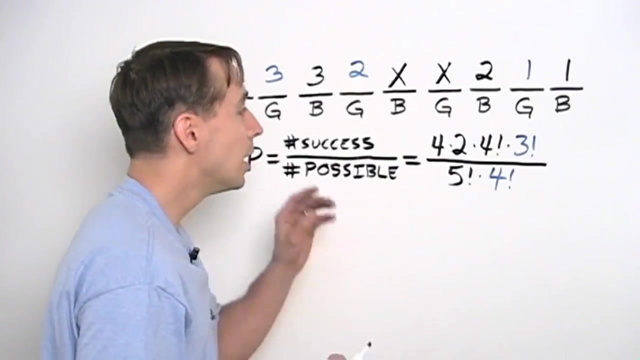 we have four factorial ways to seat the boys and then three factorial ways to seat the rest of the girls. So there we are. We've finished our two counting problems. Now you see why I like this twice as much as most counting problems. 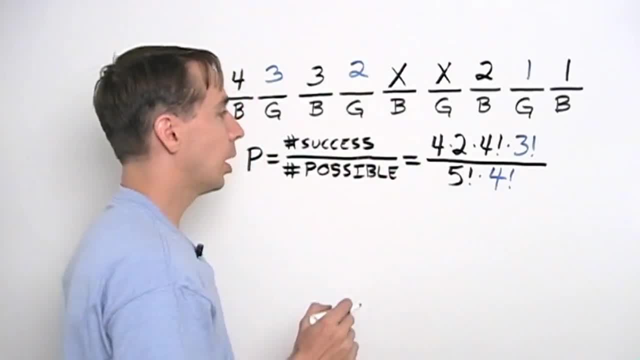 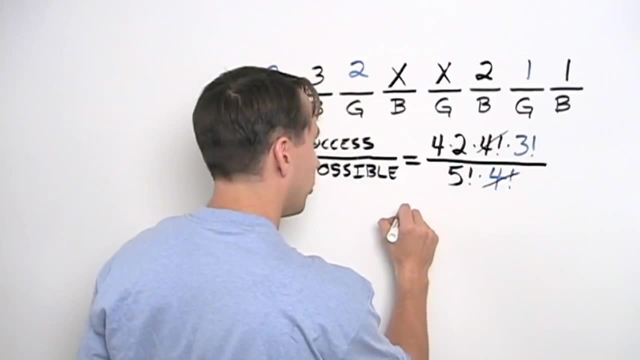 But now that we've finished the counting problem, we have an arithmetic problem. Fortunately, we can do a lot of canceling Our two. four factorials go away And let's see if we can. Oh, we still have four times two. 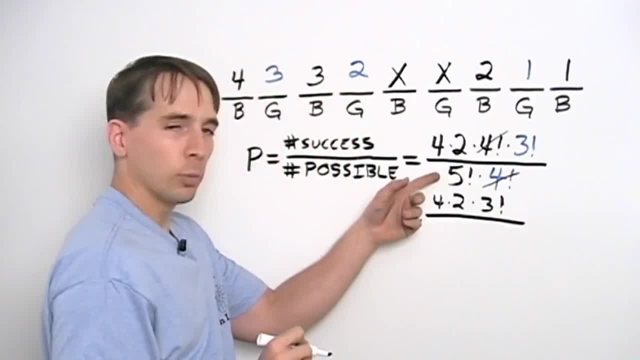 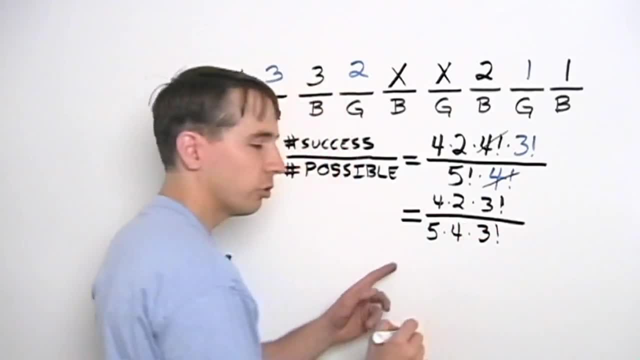 And we have that three factorial in the numerator And we can write this five factorial in terms of three factorial, because that will let us cancel some more. Three factorial is just five times four times three factorial, So now we can cancel the factorials. 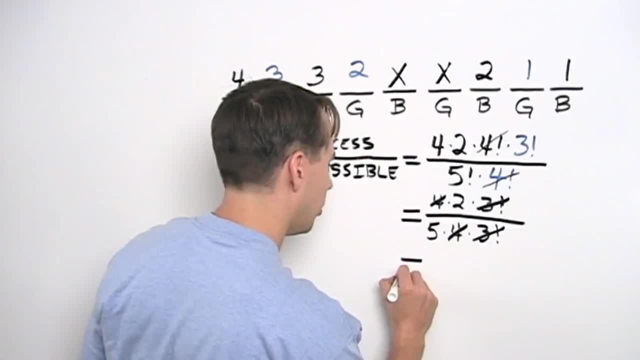 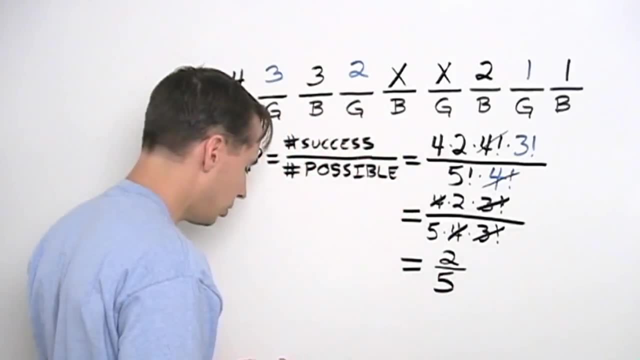 We can cancel these fours And we're left. We're left with just two fifths. It's amazing. I mean these are huge numbers. You multiply these out, you'll get pretty big numbers, But all this canceling happens and we just get two fifths.